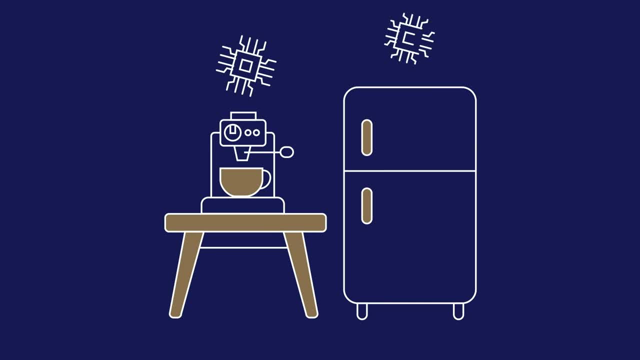 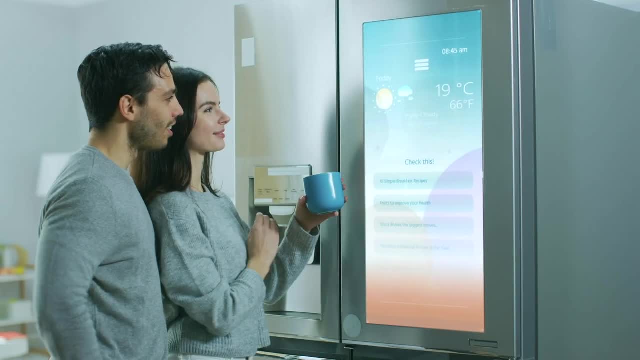 You know, the coffee maker or the fridge is going to have computing in it. So this requires new ways of sensing and new ways of humans to interact with these devices, and that is what excites me most about my research. We recognize, going forward, that one of the big challenges that 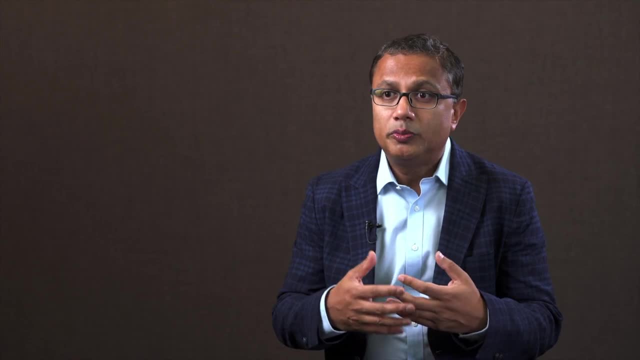 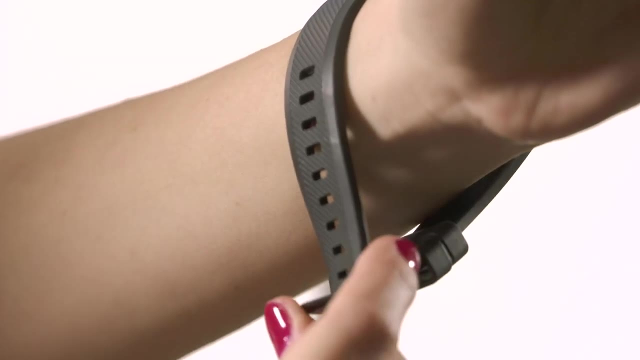 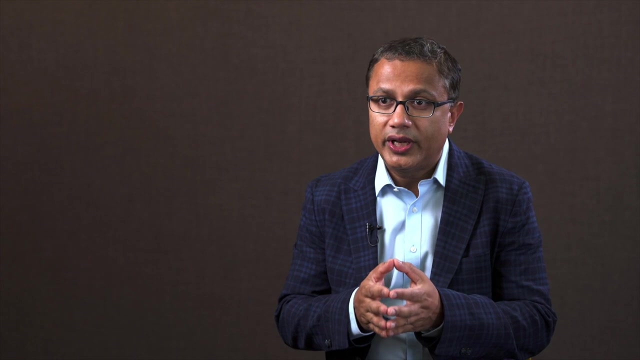 we face as sensors proliferate around us is that we just won't be able to recharge them continuously. You know, nobody likes to take, you know, a wearable device off their hand and then recharge it twice a day. So a lot of my new work is looking at the possibility of building ultra low energy wearable. 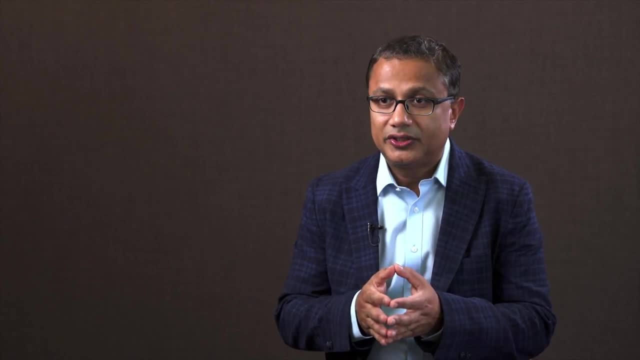 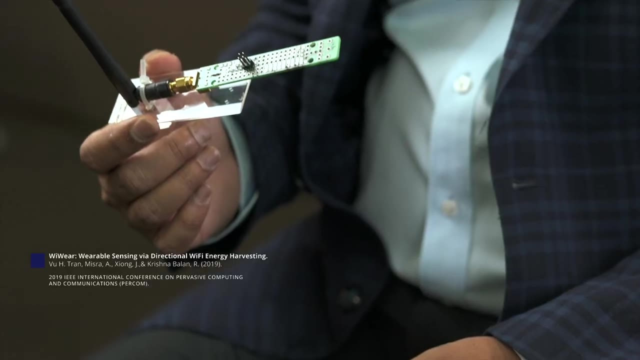 devices or battery less wearable devices. So one of the projects that I'm really fascinated by right now is this ability to build a wearable device that really has no battery and the way it's charged: it's charged by the transmissions from a regular Wi-Fi access point. Now the big innovation. 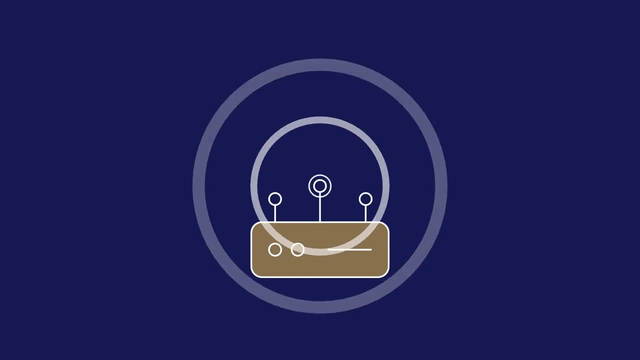 in. that is that most access point transmissions. because they're omnidirectional, they spread all around you. The amount of energy you can harvest is no more than one to two microwatts. That's too minuscule for anything realistic. However, if you're able to direct the beam using some electronic beam, 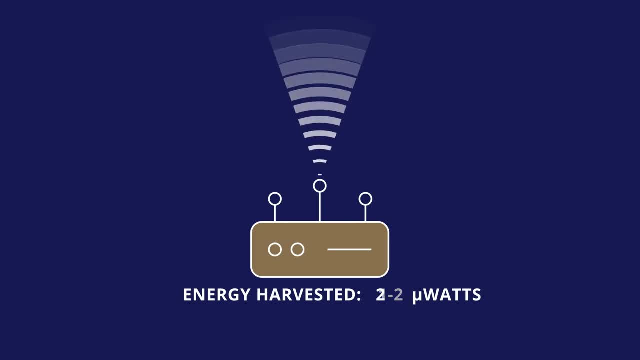 forming technologies, you're able to harvest almost hundred times more power. So what we've demonstrated recently is that we've been able to generate a lot more power than we've ever imagined. So one of the things that we've been able to do is the ability to build a wearable device. 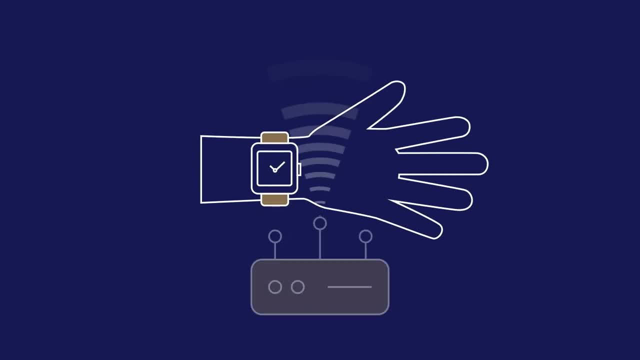 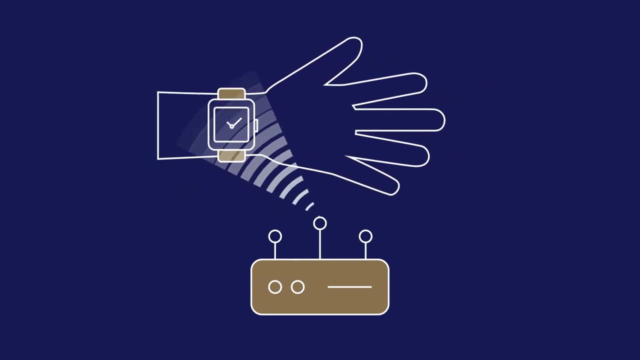 that's on your wrist, that has no battery, that is charged by this beam forming technology from conventional Wi-Fi access points, but that you can run and it can capture all the various hand movements you do in your office during the day. So, whether you're typing, whether you're having a 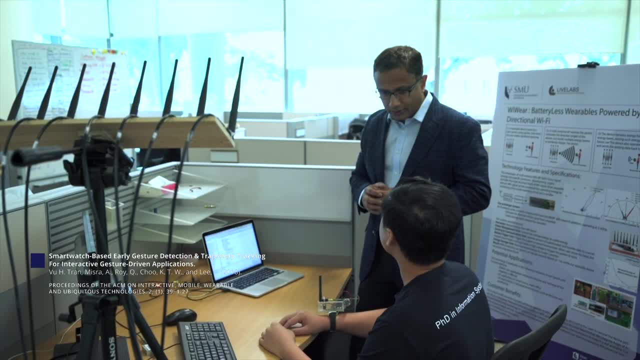 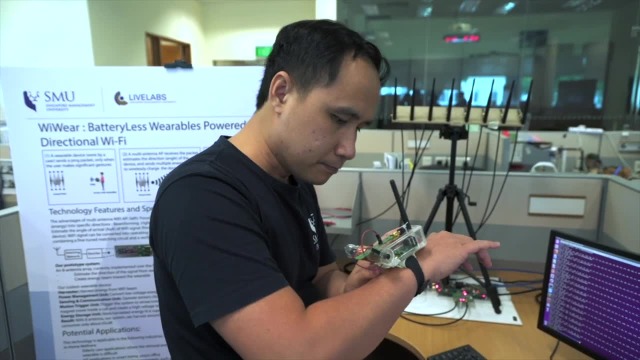 drink of water, you know whether you're sort of pointing at things on a whiteboard. you're able to capture all of these, understand human behavior without ever needing to replace the battery. So one of the projects that's actually going on and I'm very pleased that it's also being implemented in our SMU. 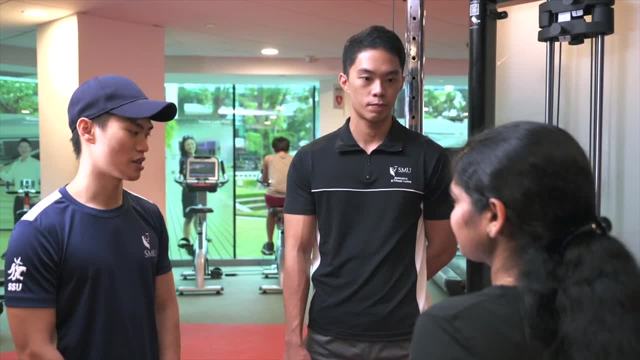 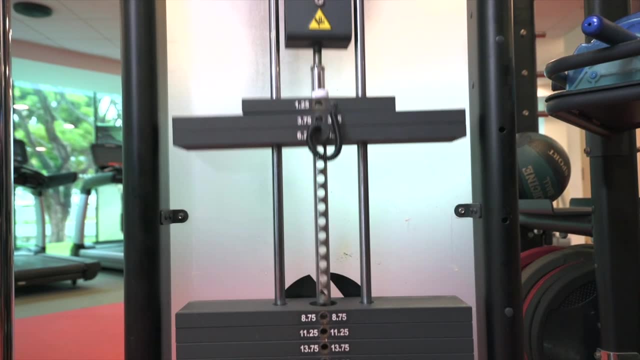 gym. So in the gym, what we've taken is- you know you have these weight stacks- we put a very simple sensor- it's a magnetometer, which is a magnetic sensor, and an accelerometer which measures the vertical up and down movement and by using the data from the simple sensor, we're able to figure out.